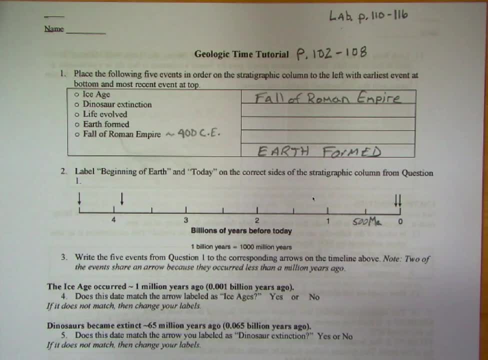 four eras and our job is to put these five events into those four eras. So that means that two of these events are close. So we can see that two events are close enough in time where they have to occupy the same arrow. So your job is to figure out which of those two events would occupy the same arrow. 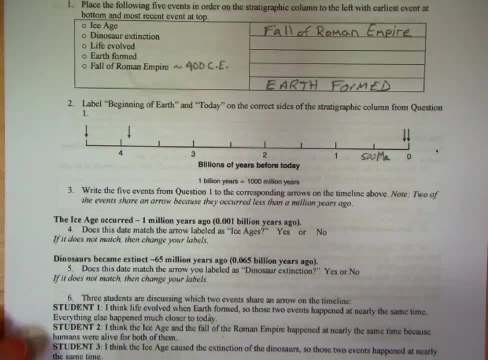 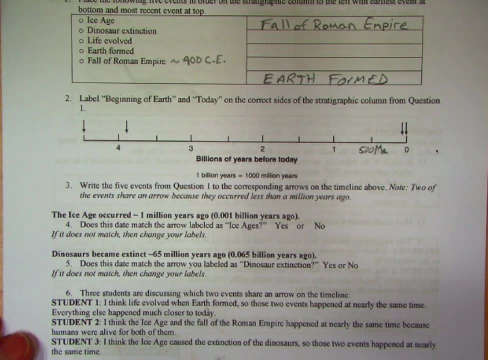 You'll go ahead and you'll look at these questions and there's some clues in here as to help, as to help you determine which of these arrows would be the two events that are closer in time. Now, as you go along here, you'll see the the general questions from students here that are: 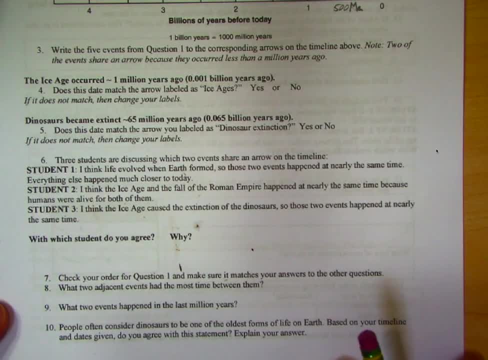 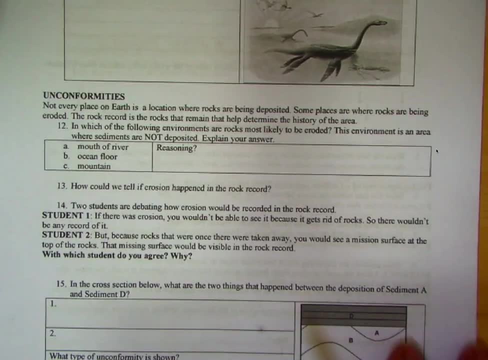 puzzled or wondering about some of these events and you can ask these in a pretty straightforward fashion On the next page. here again, this will be pretty straightforward. We get to these unconformities and these are really- remember they're sequences or spans. 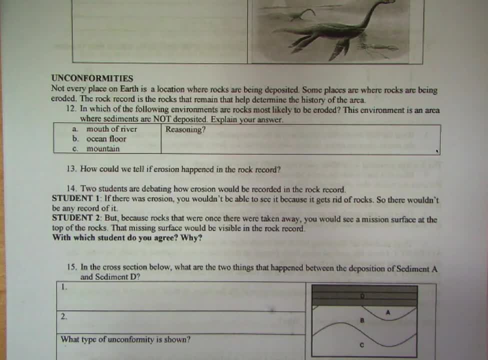 of geologic time that are not represented by physical rock units. In other words, the rocks may have been there and then were then eroded away, or maybe it was a period in time where there was no deposition at this particular point in Earth, and so there's. 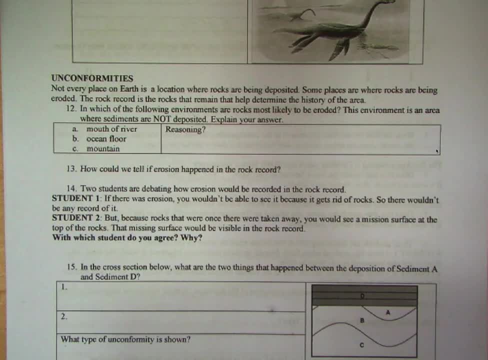 no sediment that accumulated to record the geologic events right. So again, periods of erosion, maybe periods of non-deposition, or in some cases we could even get tectonic upheaval, where there's folding and faulting and buckling of the rocks and 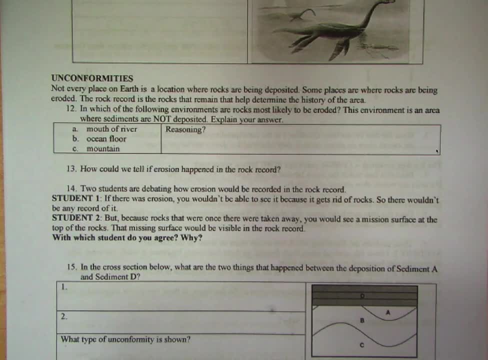 then we see we don't see deposition, instead we see the tectonic events, and then we see erosion as well. going on in there. For these unconformities, note that you'll kind of think about what would be a good place where sediment is being deposited, or maybe a source of sediment being eroded. 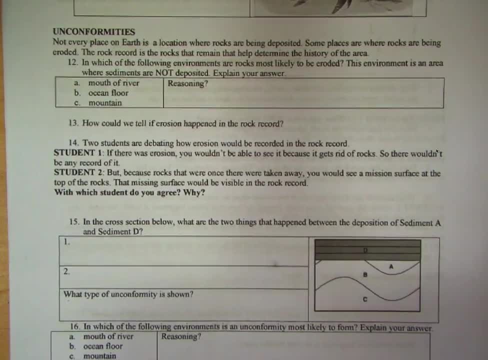 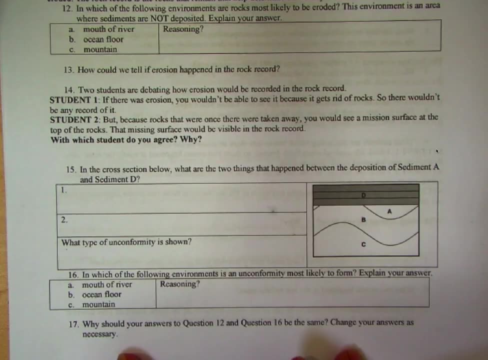 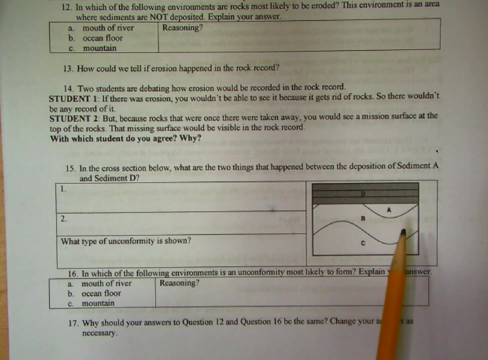 So you'll kind of go through those And remember I discuss all these in my video lectures online as well. Now for question 15, here we're looking at a particular type of unconformity where the older strata C, B and A have been folded and buckled by some event, some tectonic upheaval. 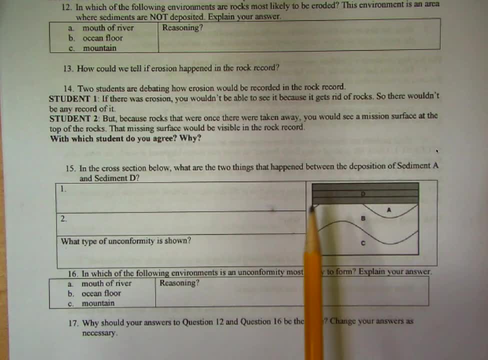 that did not affect the younger units here, D So this line here is one of those erosion events which is probably one of those tectonic upheavals. Okay, So we're looking at a particular type of unconformity where the older strata, C, B and A, have been. 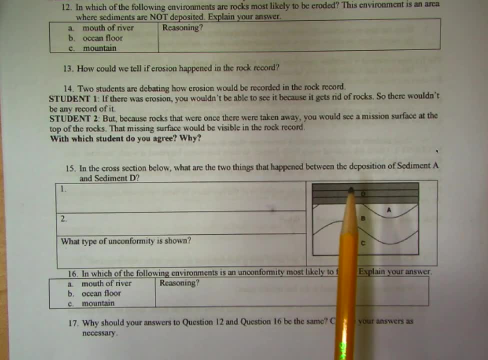 folded and buckled by some event, some tectonic upheaval, events, because whatever event folded and buckled, these did not affect letter D. So this type of unconformity would be an angular unconformity, So angular unconformity. you would place that right there. 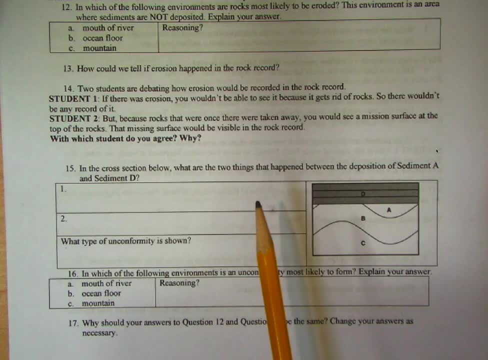 And then you can kind of talk about two different things, like you know, for example, what two things might have happened. Well, sediment A, B and C, they were deposited, they were lithified, and the other thing that 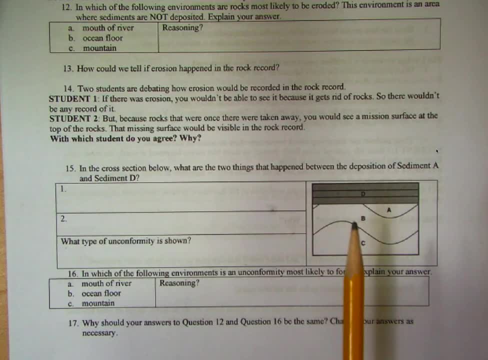 could happen: they were folded or they were deposited folded And then The erosion event occurred and then we have deposition of D. So there are several things that are happening before D is deposited there, right, So you can write those in here. 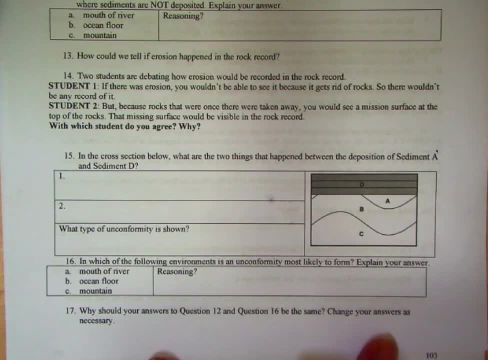 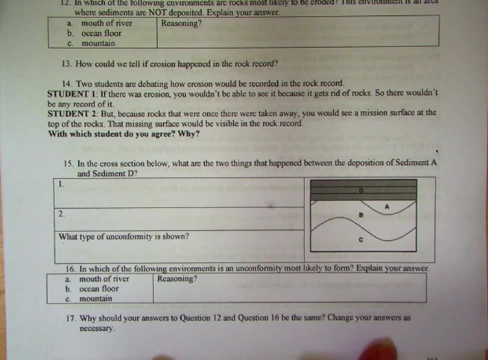 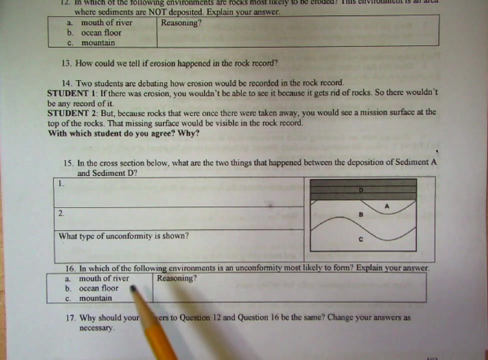 So you can just kind of spell out two different ones there. Question 16 kind of follows the same idea as question 12 up there, where what environment you think would be an unconformity? where there's no deposition or maybe erosion, And so obviously river mouths and ocean floor are always accumulating sediment, whereas 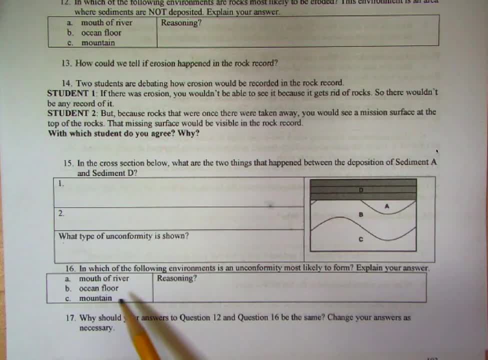 the mountain would be a source of sediment, so that would be where erosion is occurring. Probably the mountain would be the best choice here, and then you would give some reason as to why these other two would not be places of unconformity. Again, like I said, question 16 is similar to question 12.. 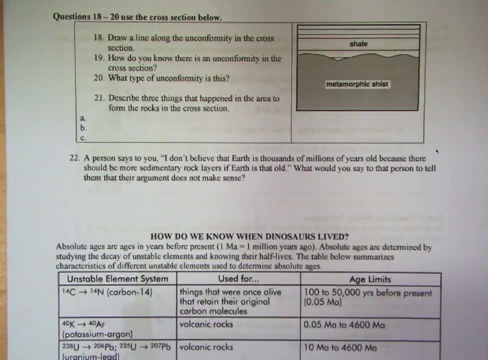 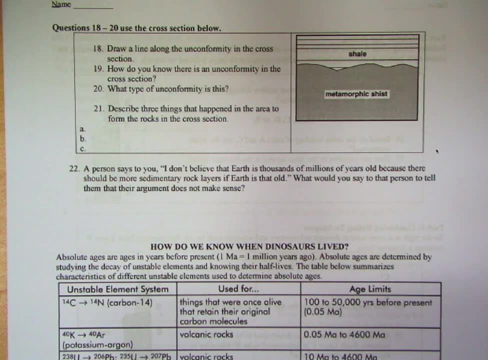 Now you can kind of answer this question as well. Continuing on with unconformities here for questions 18 through 20 or 21, here we're seeing: in this case we have a crystalline basement, So remember, crystalline basement. 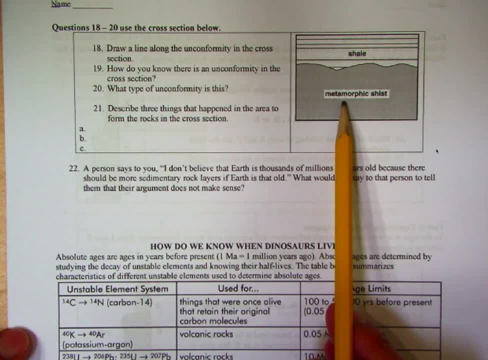 Where a crystalline basement is either a metamorphic rock or a plutonic igneous rock, like a granite, some sort of granitic rock or, in this case, a metamorphic rock. What granite, plutonic rocks and metamorphic rocks? what they share in common is that they 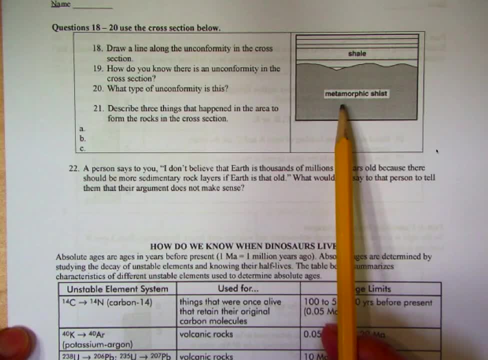 both formed at depth right, So not on Earth's surface, whereas shale- we know shale forms up here on Earth's surface. That's a sedimentary rock And so this contact between the shale and this metamorphic rock, that's a sedimentary. 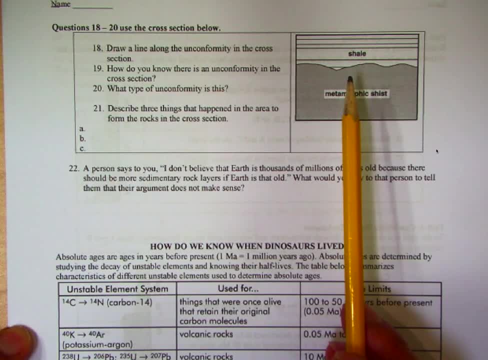 rock that's a metamorphic crystalline basement is an unconformity, a time gap, because you need time to erode whatever was above the metamorphic rock, expose it at the surface and then put the new shale on top right. 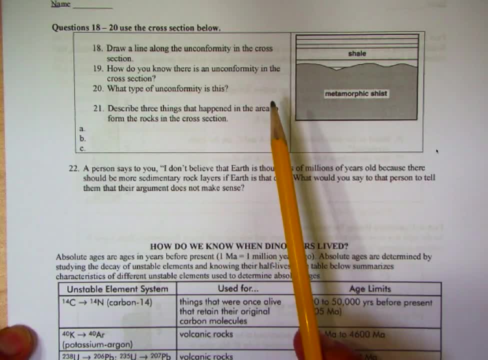 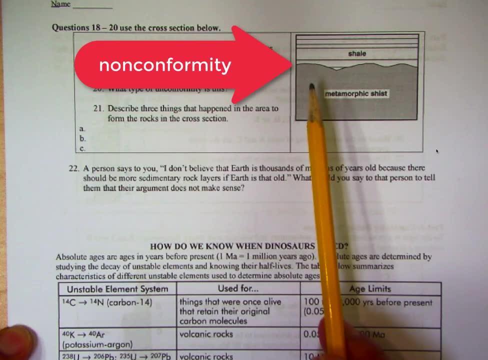 So that's a time gap. So again, you would describe this one And remember this type of unconformity. in my videos I call a nonconformity- nonconformity. Kind of think about this question too. 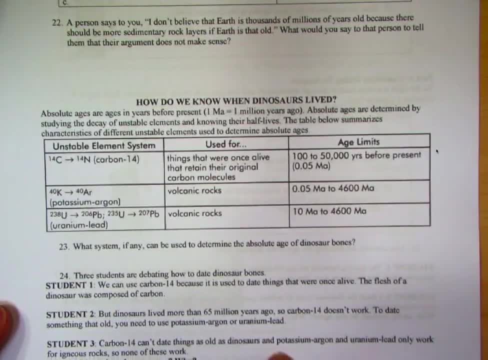 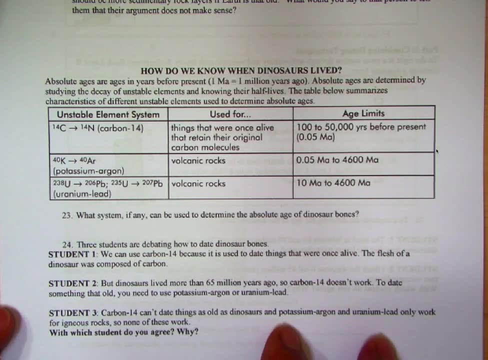 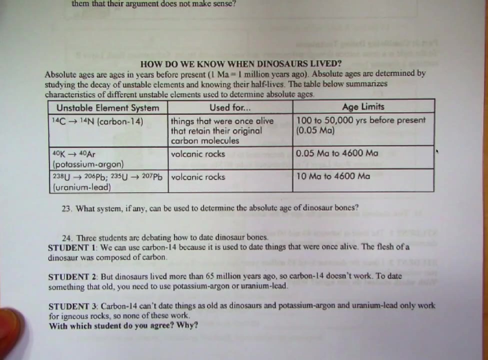 Give me some notes here. We'll take a look at those. Okay, Let's move on to this absolute time, or the numerical time, where we use isotopes, atoms, atomic clocks, radioactivity, to date, geologic material. So for this one, we're looking at three different isotopic systems. 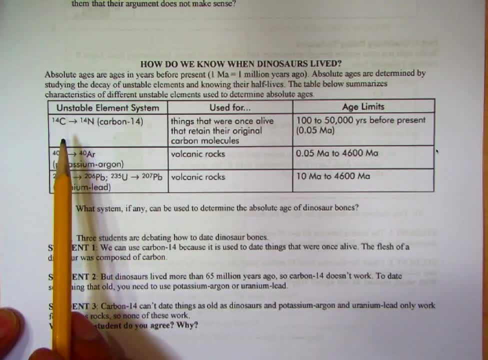 Remember, these are the parent-daughter pairs. They're isotopic clocks, atomic clocks that keep a constant rate of time by decay. And we have the carbon-14 and nitrogen-14, potassium-argon system And there's really two here in the uranium system. 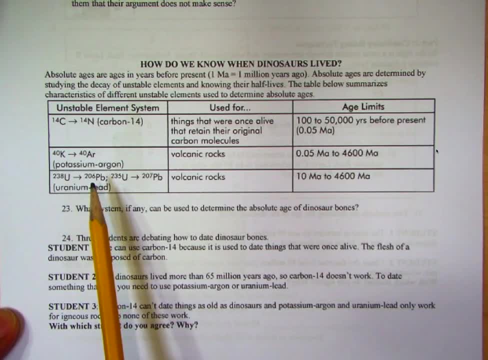 There's 235, 207, and 238, 206.. So these are all independent atomic clocks that are keeping track of geologic time in a closed system And so we can use these to date rocks And, you can see, mostly for the potassium-argon and the uranium systems we can use them for. 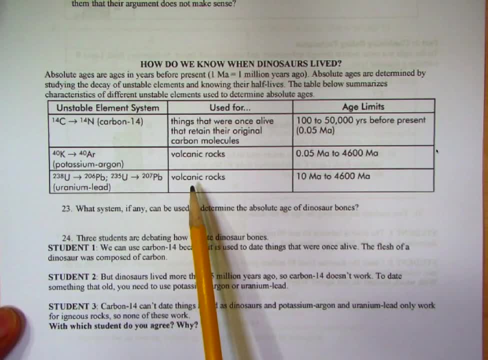 volcanic rocks and also igneous plutonic rocks like granitic rocks. But note that for carbon, carbon can only be used for something that was once alive. So we can use these to date rocks And, you can see, mostly for the potassium-argon and the uranium systems we can use them for. 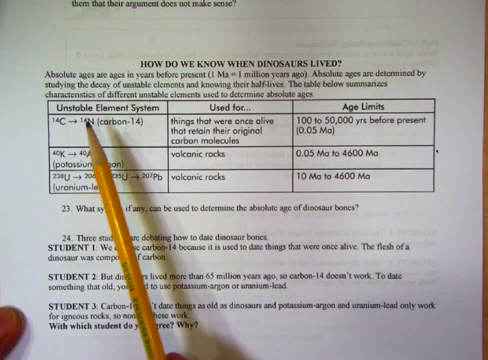 volcanic rocks and also igneous plutonic rocks like granitic rocks And, you can see, mostly for the potassium-argon systems. we can use them for something that was once alive. So in my video lectures I talk about how carbon-14 is being continuously made in the 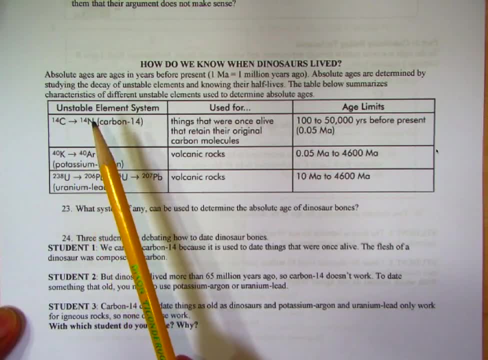 upper atmosphere And then over time it decays in nitrogen-14.. So as long as the organism is alive, it's getting its constant supply of carbon-14.. As soon as the organism dies, the system closes and the atomic clock begins to tick. 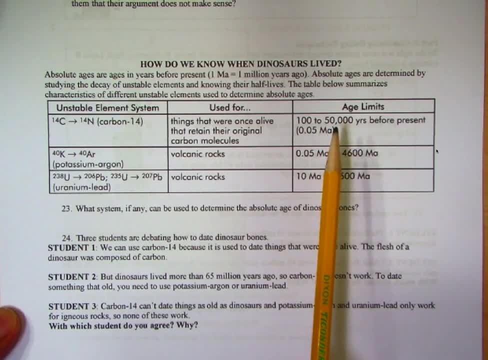 And so note that here we really can't go anything older than about 50,000 years, So we can't really date anything over than 50,000 years, And also that material had to have naive probabilities, And so we're going to go back to Adam's expression. 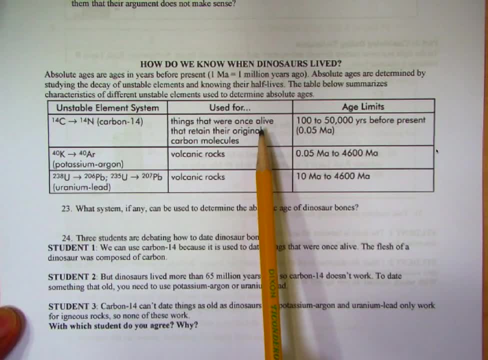 There's another host of incidents where we can kind of count on natural, natural, natural situations to deteriorate on. that was when the Bern tutorial came on. once been alive like a plant or an animal, right that was accumulating carbon through either photosynthesis or by eating organic molecules it was. it was getting its supply of carbon. 14. 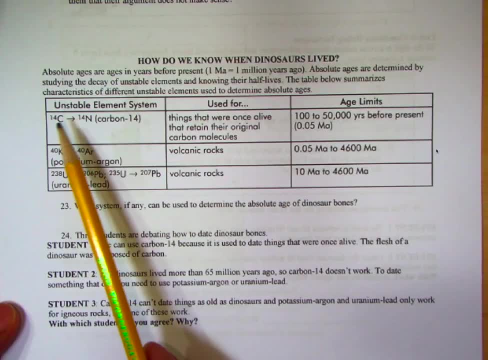 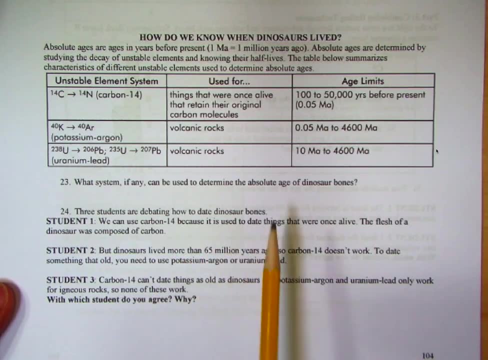 but then when it dies, it's no longer receiving 14, so the system closes and we begin to have a parent-daughter atomic clock there. look at these questions, remember, for dinosaur borns? dinosaurs lived or went extinct around 65 million years ago, so obviously we can't use carbon 14 because we 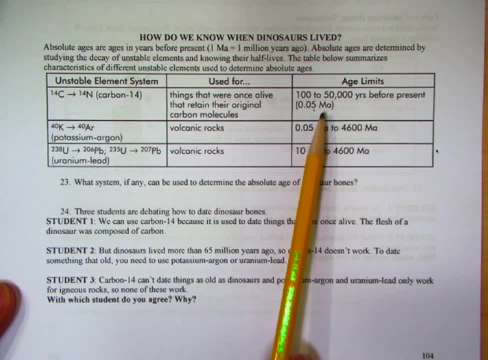 can't we? it only goes out of, goes back to 50,000 years. we cannot use these because uranium and potassium argons are only used for volcanic rocks or or igneous plutonic rocks, right? so kind of think about these questions and then you can pick out what answer you want to choose there for part two. 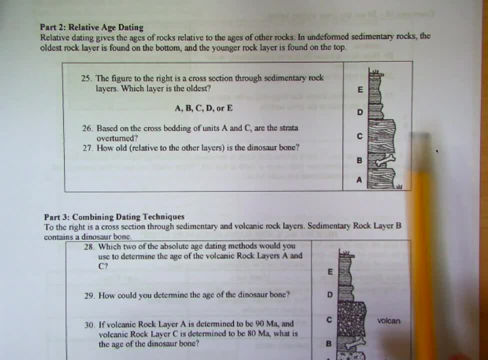 you here. we're looking at a cross section with some sedimentary structures. remember in in sedimentary rocks about i talked about these cross beddings, and cross beddings are like when sand dunes are being formed, either on a coastal dune, or ripples are being formed, and we always notice when they're. 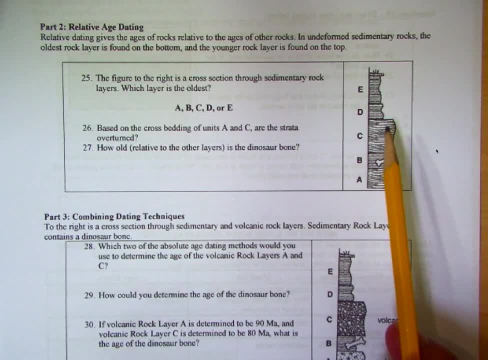 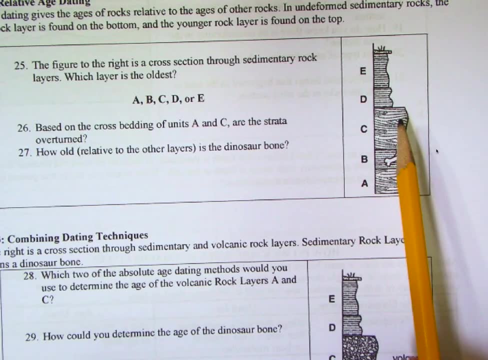 being formed is that the the tops of these dunes are being truncated. so if we look closely at this section here, we see that these cross-bedded four sets or dunes come to an end right there, so they're being cut by the next layer above it, which means that these 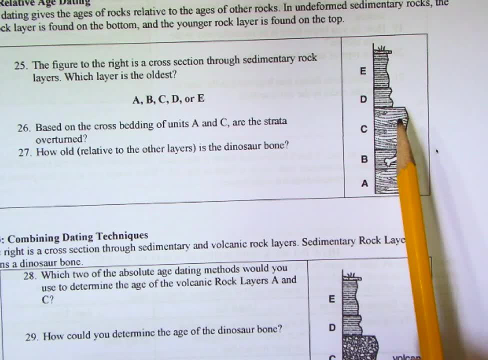 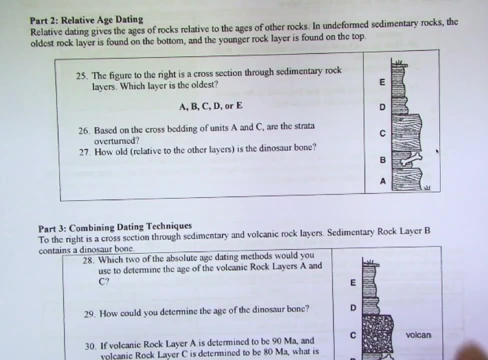 have not been overturned. they're in their proper position. these units are going from older on the bottom to younger on top, so the sequence is in order. so that's that question here. based on the cross-bedding, well, we can see that it's not overturned. all we can do in this section here. 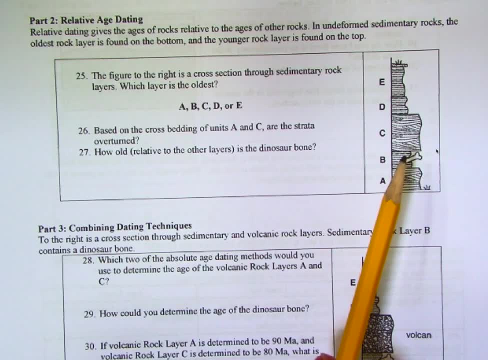 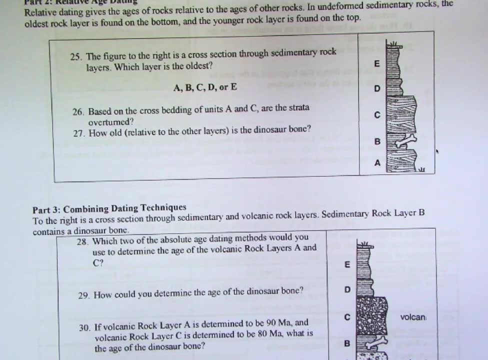 we can't date the dinosaur born directly, just as we proved in the previous question, but we can figure out the ages of units that are going to be in the next layer above it, so we can see that it's below and above it. so, in other words, in this case here in terms of relative time, relative to the 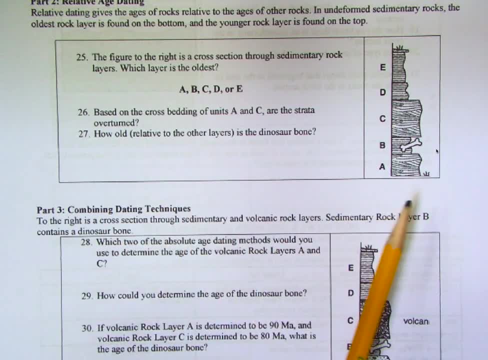 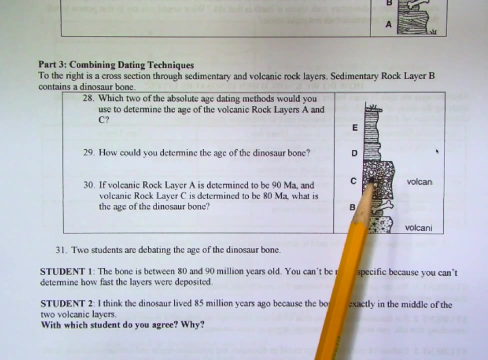 others. we know the dinosaur bone has to be younger than unit a but older than unit c, just because it sits in between right now. for this next one, it's kind of the same idea, but here we have some lava flows and we can date these radiometrically. in fact, they've done it right here. we don't know the. 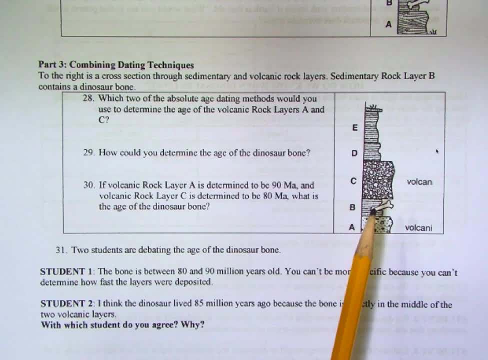 exact age of the dinosaur bone, but we can bracket it between the units that are going to be in the middle and above it so we can get a range for this. and we won't get it exactly, but we can get a range. so you can kind of answer these questions there and then again you can answer the the student. 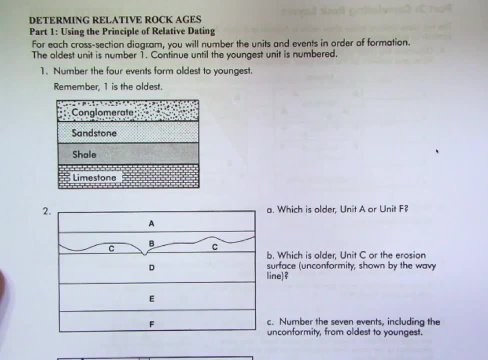 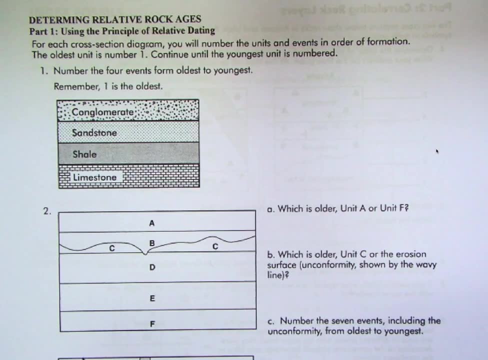 questions down below this next one we're going to start playing with is these relative geologic time puzzles, and one of the principles that we use is the principle of superposition, and obviously here we're seeing limestone, shale, sandstone conglomerate, which limestone would be the oldest, based on the principle, principle of superposition, whereas conglomerate will be the. 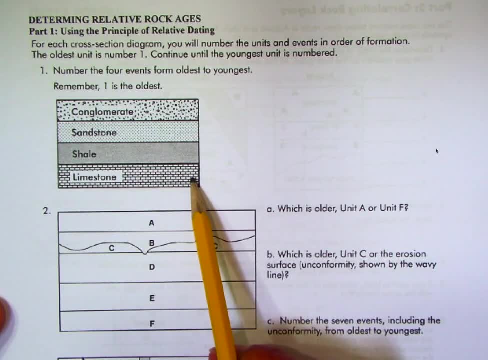 youngest here also. what this is showing is that we know that limestone forms in deeper marine waters. shale is kind of a outer continental shelf to shelf environment, so it's shallower marine waters and sandstone we know is is either a continental shelf or a shoreline coastal. 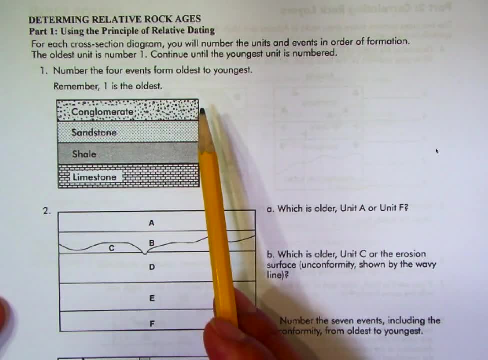 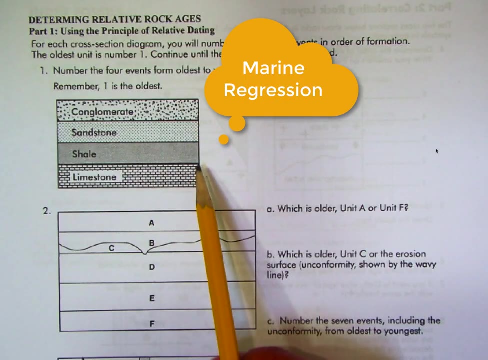 environment and then we know conglomerate forms in rivers. so this is showing over time where sea level was much deeper here and then sea level got shallow. so we call this a marine regression, marine regret, and i talked about these a little bit in lecture, so- and i do in my video lecture as well, so this 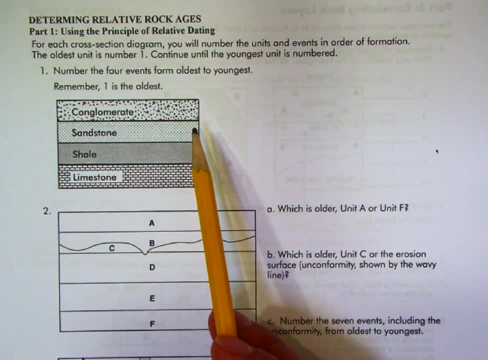 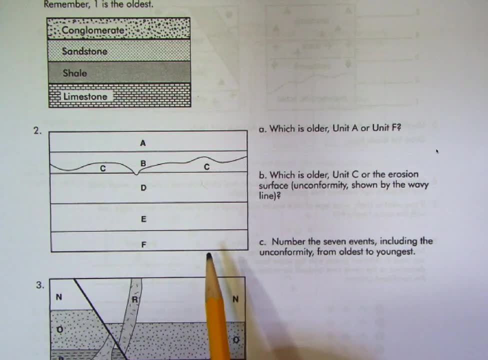 would be a marine regression, remember. the other one would be a transgression for question two. here again we're doing the same idea, kind of this geologic puzzle. we know that, based on superposition, f would be the oldest unit, so we call that number one. then number two would be a unit e, because that's the 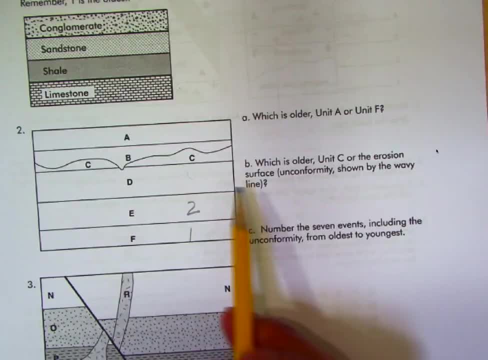 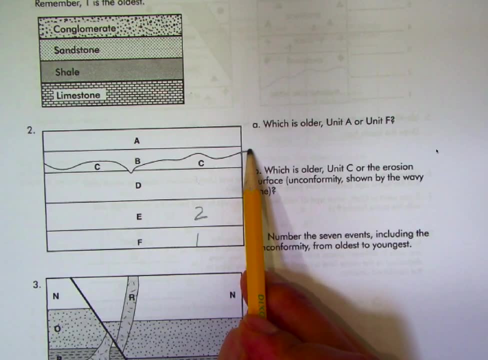 second one. you can see that we got three, four, but remember this, this, this erosion event, right here, that's, that's an event we have to number and that's an unconformity. in this case, when you see parallel strata below and above the unconformity, note that they're parallel. 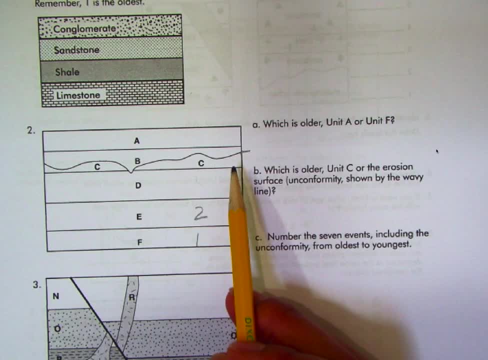 it's not going to be angular conformity. we don't have any crystal embasement here, so it is an event. but between parallel sedimentary units we call this a disconformity. so that's our third type of unconformity disconformity. so it would be one, two, three and then we have unit four would be. 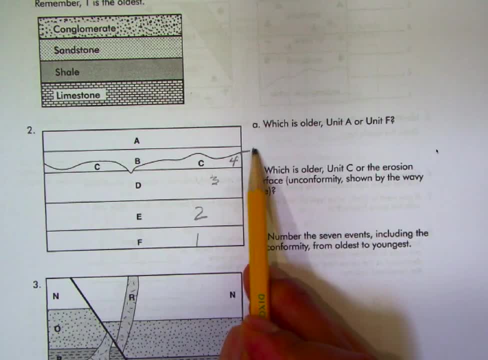 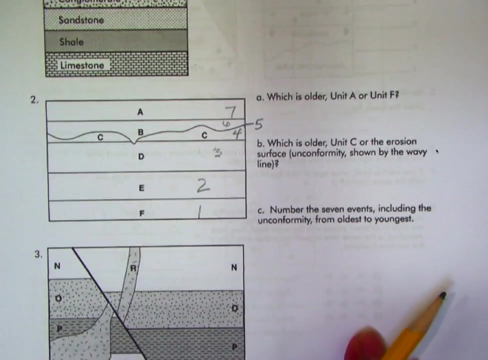 c, here the, the disconformity is five, and then we have six and seven for b and a. so that would be the relative sequence or order of events where one is the oldest, seven is the youngest. right, then you can answer these as we go along here. we haven't talked about geologic faults here, but 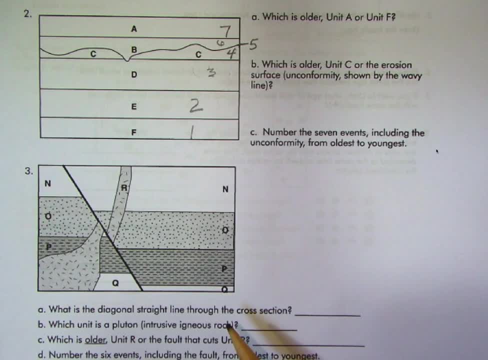 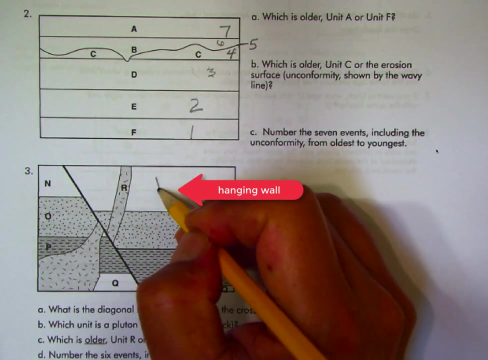 remember, a fault is a fracture in rocks where there's displacement or slippage. so obviously here there's some slippage. and when we talk about faults here here's a fault plane and the, the, the block above the fault plane, is always called the hangar. 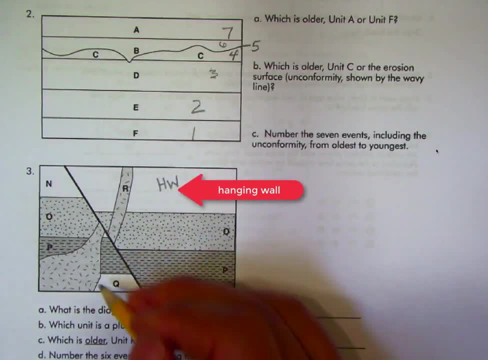 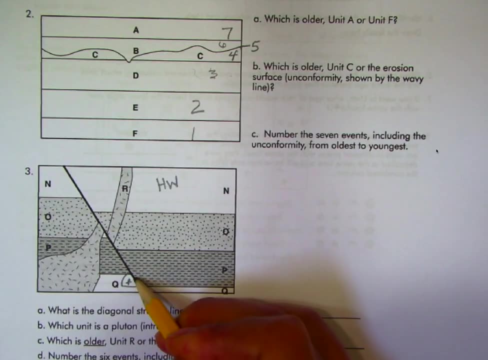 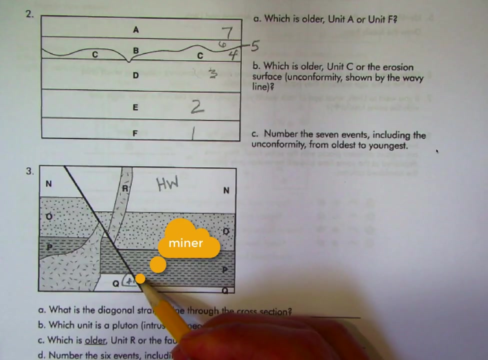 wall, block the hanging wall because, yeah, you can hang. if you, if you drill, made a mine shaft in here and you can stand in here, you, you, would, you, would. you can hang something from the hanging wall, right, that's why it's called hanging wall, so miners would use those terms and then, uh, same time, uh. 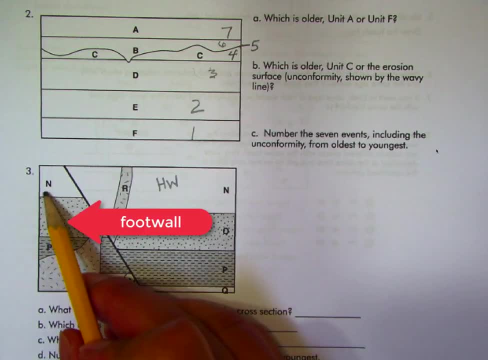 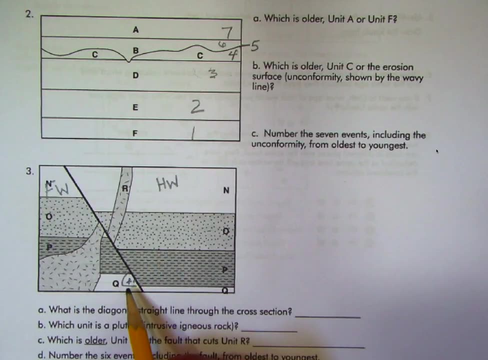 this bottom area here is called the, the footwall block, fw for footwall, and that's because you could walk. in fact you can see the miner down here. my little cartoon of a minor is walking down here on the foot wall right, and so you can. you can literally walk on the foot. 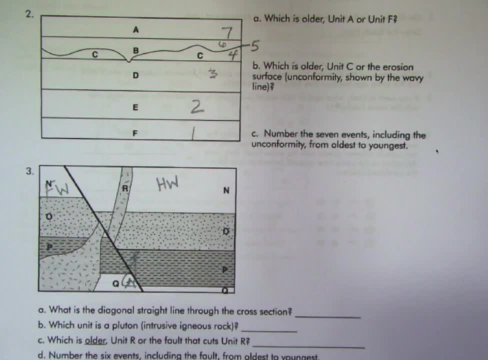 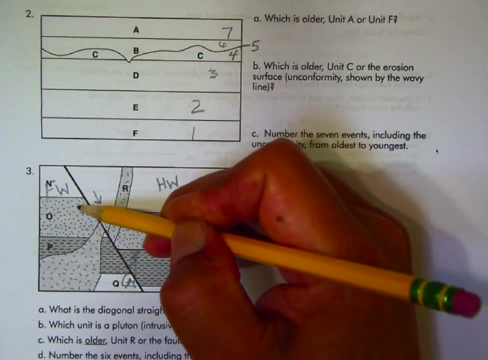 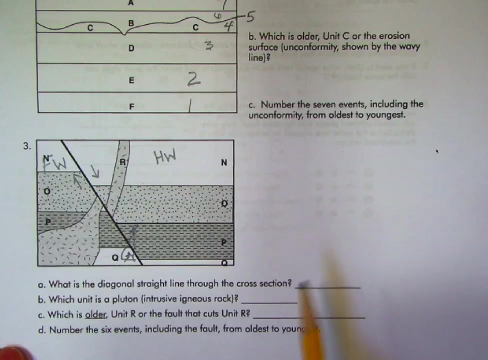 wall here. so we have we have foot walls and hanging walls, and so the fault where the hanging wall moves down relative to the foot, to the foot wall, we call that a normal fault. this is a normal fault, and so there's probably a question about that. here we're going to, we're going to invoke: 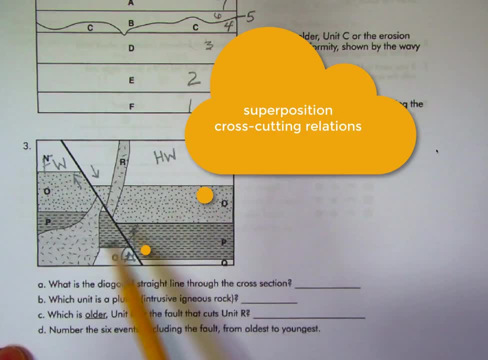 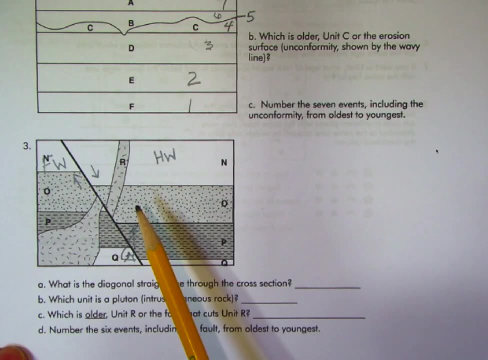 two principles: the principle of superposition and the principle of cross cutting relations. and so again, we want to number the events here from from oldest to youngest, and obviously the oldest would be q and the youngest is probably going to be this fault, because the fault seems to cut everything, and we know that r intrusion r here has cut through n. so r based on the principle 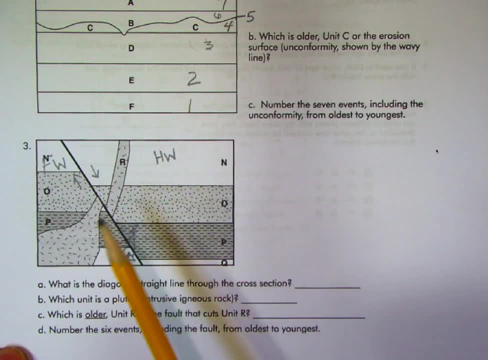 of cross ten relations has to be younger than n. so it's a classical argument of superposition, which is the reason why we have to call it wrangling the firebox, which is the principle of superposition, which is the problem of superposition. So try to figure out the relative orders. 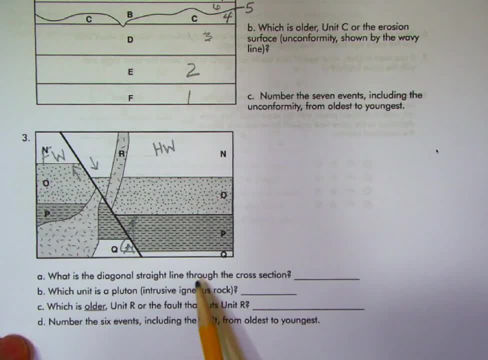 of these events here. So obviously that's a fault for letter A and this Pluton is letter R And which is older, unit R or the fault that cuts it. So, based on the principle of cross-cutting relations, the fault cuts the Pluton R.